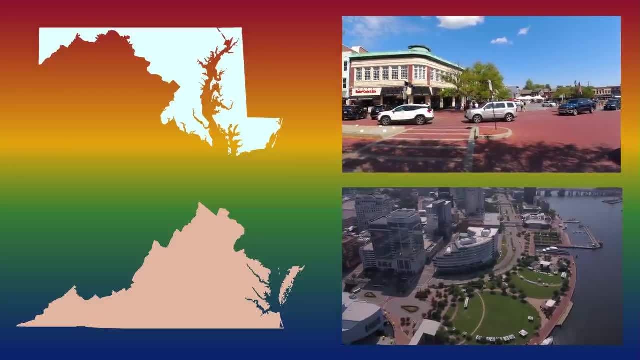 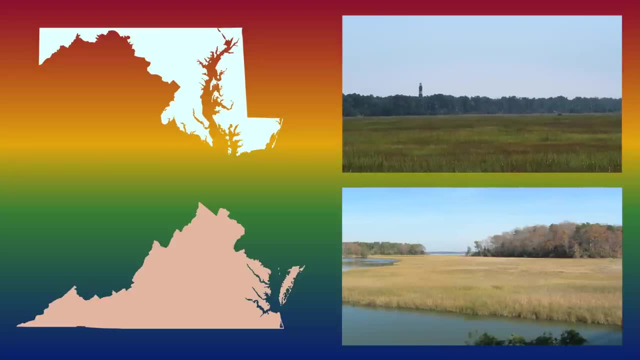 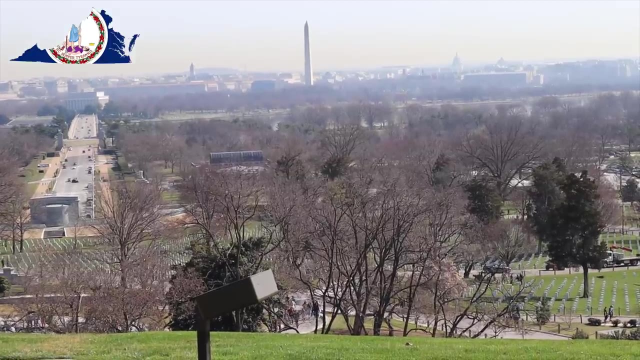 in the winter months, but both have quite humid springs and summers. if you can't handle humidity, Yeah, don't move to Maryland or Virginia. Both have a topography that's diverse, with sandy dunes and low marshlands near the ocean to gently rolling hills in the Piedmont region. 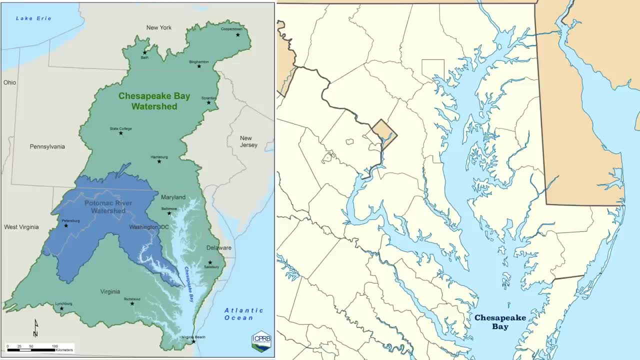 to the aforementioned mountains. out west, the Chesapeake Bay, The largest estuary in the country, splits up both states. On the east side of it is the Delmarva Peninsula, which includes both the eastern shore of Maryland and eastern shore of Virginia. 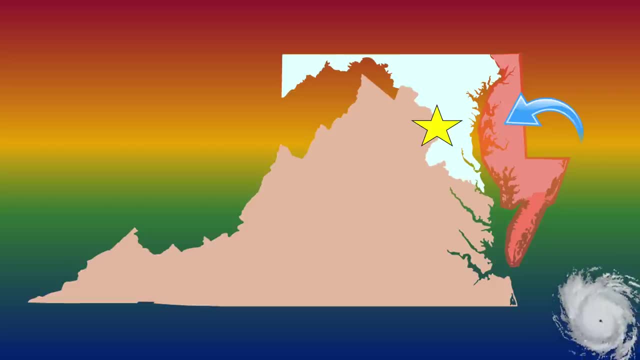 The eastern shore of both states is more rural and flat and more vulnerable to hurricanes and rising sea levels due to climate change. Now, the eastern side of both states is more rural and flat and more vulnerable to hurricanes and rising sea levels due to climate change. The eastern side of 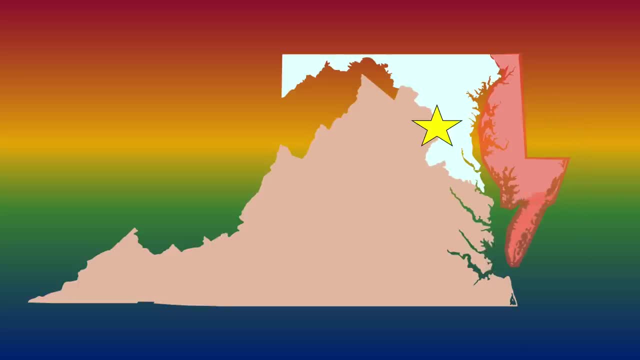 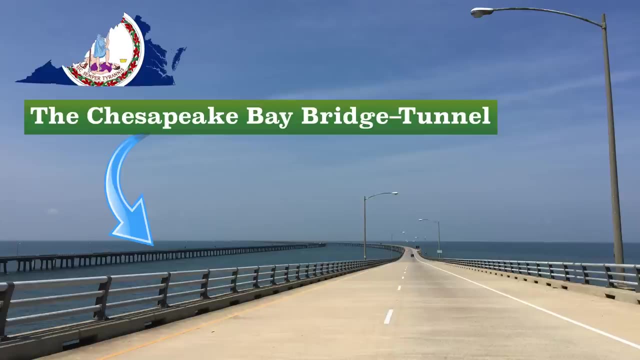 climate change. Both states have just one highway that links the eastern shores to the rest of each state. The Chesapeake Bay Bridge Tunnel links Virginia. It is one of only 12 bridge tunnel systems in the entire world. The massive Chesapeake Bay Bridge connects. Maryland, and it's freaking, busy and always backed up, especially during the summer, which is why Maryland's government has considered creating a second bridge that crosses the Chesapeake. The median age in both is nearly identical. Both states have two of the lowest. 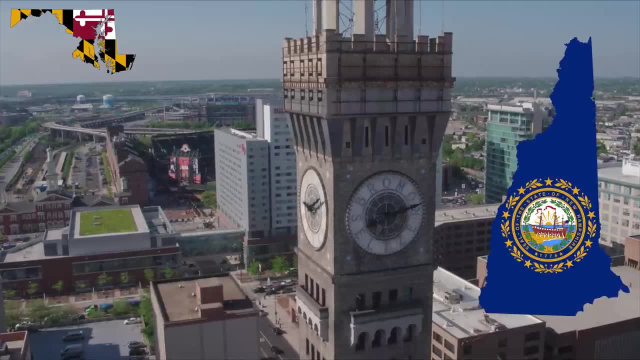 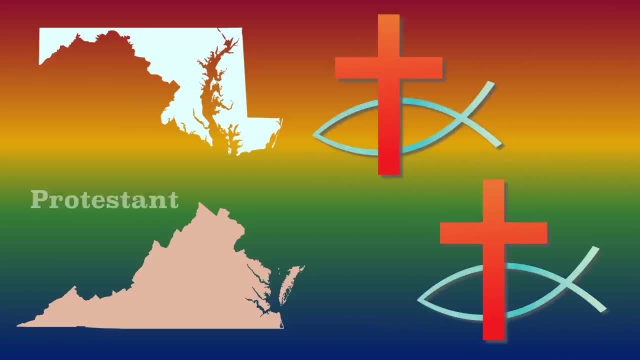 poverty rates in the entire country, Only New Hampshire currently has a lower poverty rate than Maryland. The biggest religion in both is Christianity, specifically Protestant, although Maryland has quite a bit of residents who identify as Roman Catholic. More on why that is later in this motion picture. Both have lots of historic sites. If you're a regular 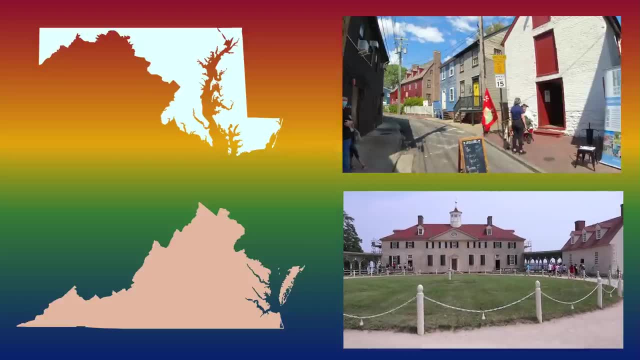 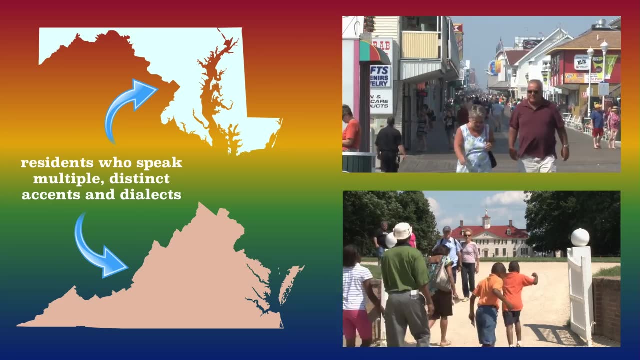 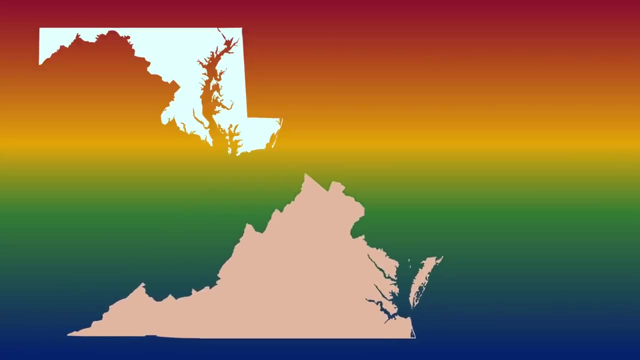 viewer. you'll know why. First of all, thank you. And second, you would love all the preserved history in both. Both have residents who speak multiple, distinct accents and dialects. So what about differences? Well, first of all, Virginia is bigger in land area, About four times bigger actually. Virginia also. 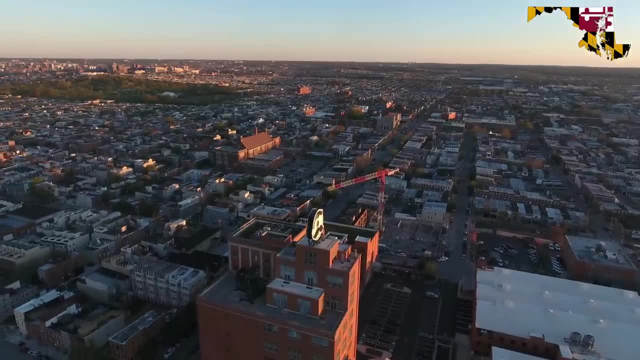 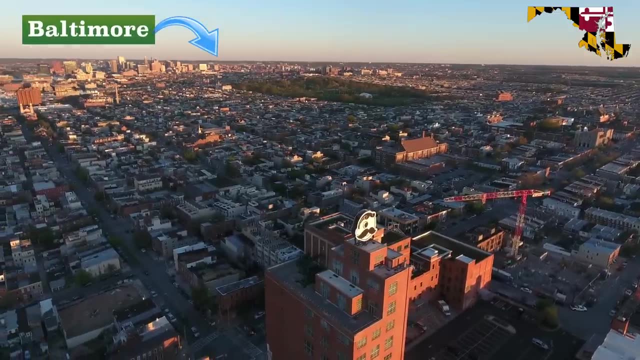 has more people. That said, Maryland has a higher population density and only four states have a population density. So if you're a regular viewer of my channel, first of all, thank you. Maryland's largest city, Baltimore, also is much bigger than Virginia's biggest city. 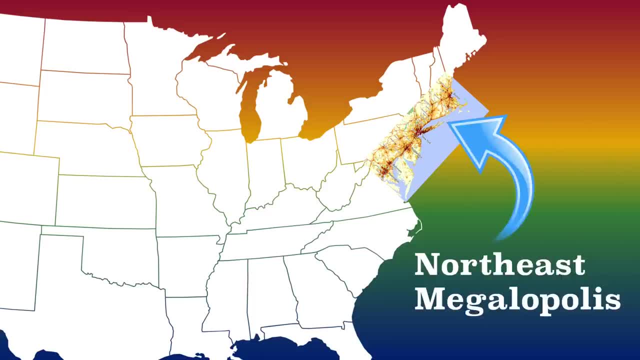 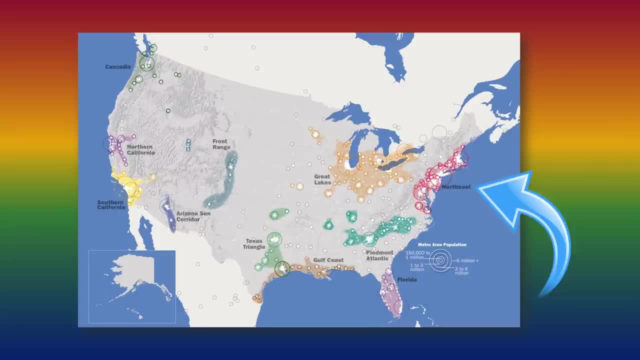 Virginia Beach. Maryland is completely part of the Northeast Megalopolis, a part of the country that contains more than 17% of its entire population, or some 50 million people on less than 2% of the country's land area. The cost of living. 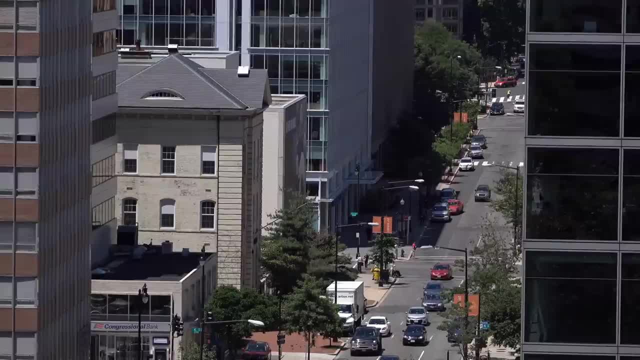 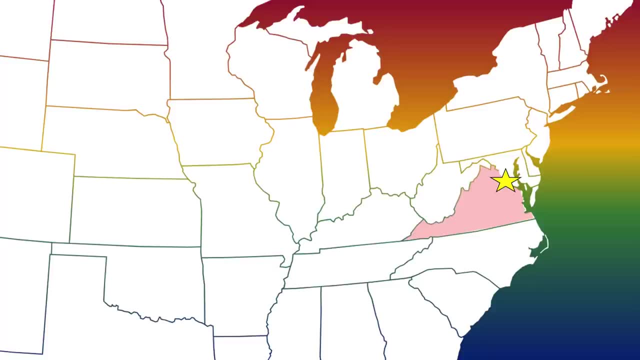 is higher in Maryland overall. That said, around the District of Columbia it's all expensive, For real Virginia borders more states, In addition to bordering the District of Columbia, which is not a state of course, and Maryland Virginia also borders West Virginia, Kentucky. 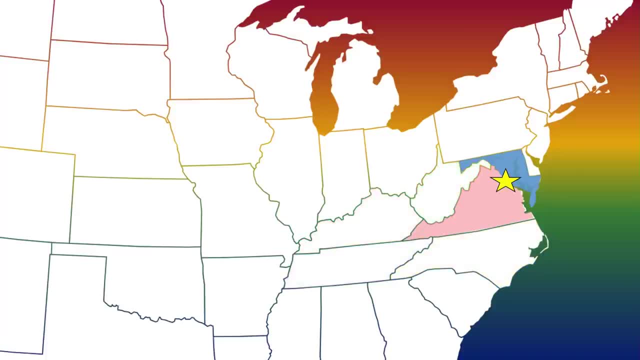 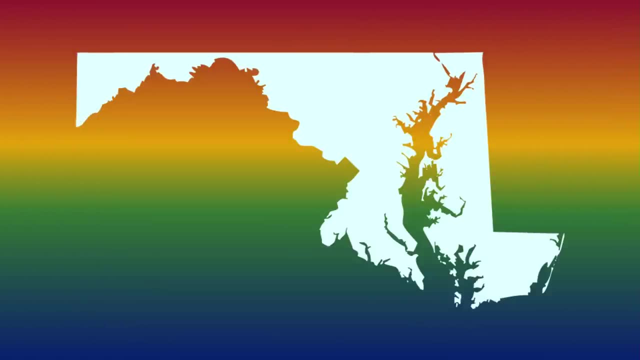 Tennessee and North Carolina. Maryland also borders Pennsylvania, Delaware and West Virginia, And now might be a great opportunity to talk about how Maryland is totally the weirdest shaped state in the country. What the heck is up with that, anyway. I mean, it's almost. 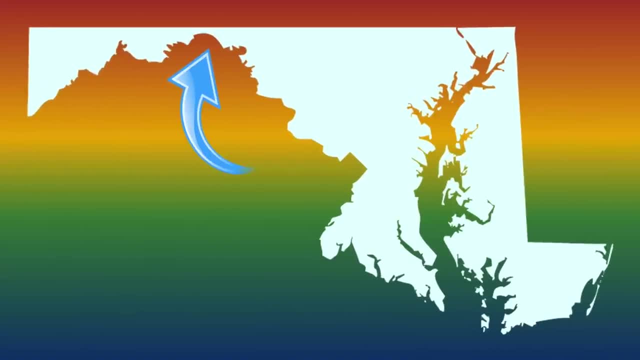 broken into two right there. By the way, this area is often called Maryland's Narrow Waist or Skinny Neck. At its narrowest point, there is less than two miles of Maryland between West Virginia and Pennsylvania. Well before we get into how Maryland got its crazy. 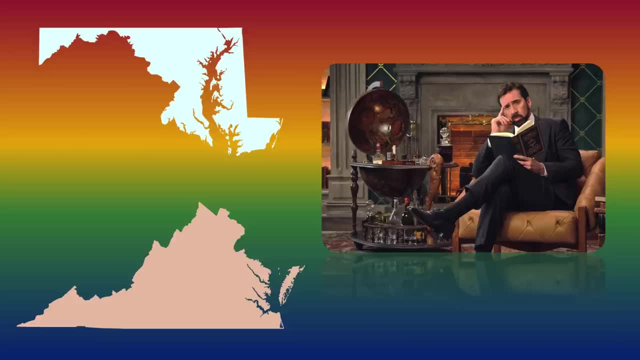 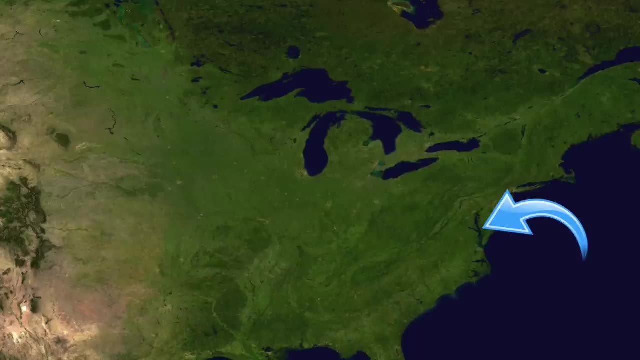 shape. let's just get into the history of both states, shall we? We shall Well, good we shall. indeed, Humans have lived in the area of modern-day Virginia and Maryland for thousands of years, before European occupation, And so, as we've seen, Maryland has been a great place to live, And so 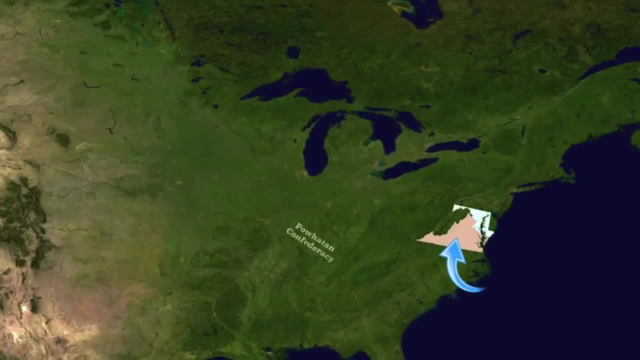 as we've seen, Maryland has been a great place to live And so, as we've seen, Maryland has been a great. eastern modern-day Virginia was dominated by the Powhatan Confederacy. However, several other American Indian tribes are native to the area, including the Tutelo and Saponi Catawba, and 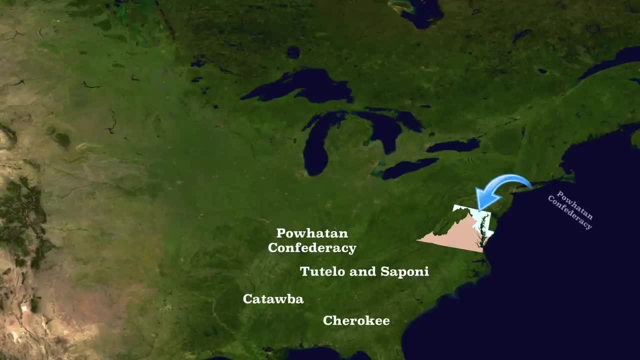 Cherokee. Meanwhile, modern-day Maryland was also home to the Powhatan and Tutelo and Saponi, but additionally the Nanticoke, Lenape, Susquehannock and Massawamek In 1607, the English. 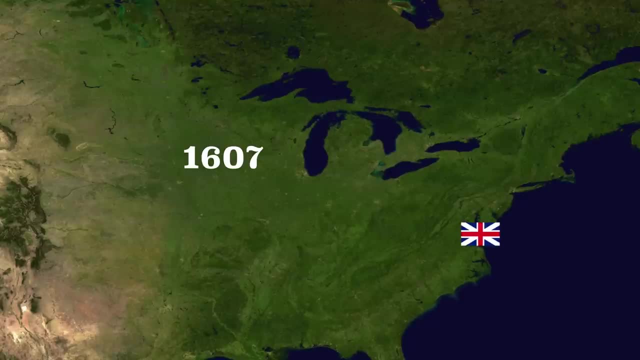 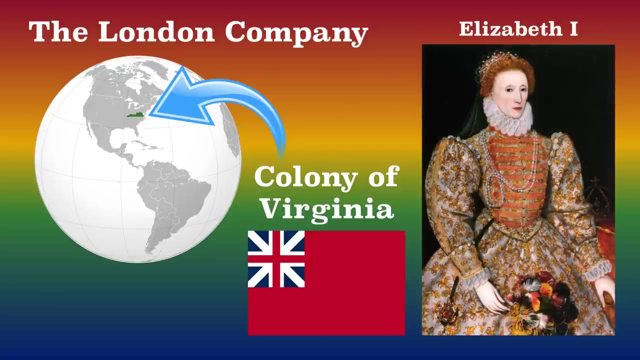 came over- In fact, that's why I'm speaking English to you right now. The London Company established the Colony of Virginia, named after Queen Elizabeth I of England, who was also known as the Virgin Queen. Eh, Eh, Anyway, the Colony of Virginia was the first permanent English. 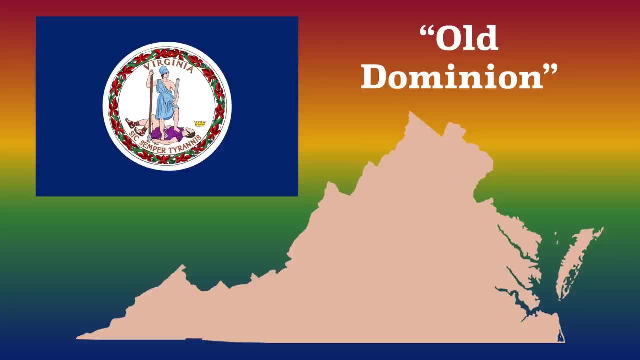 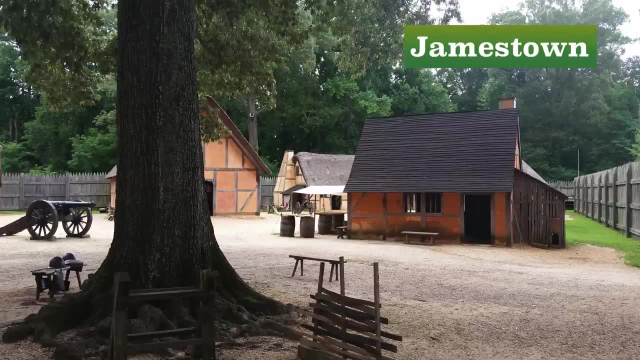 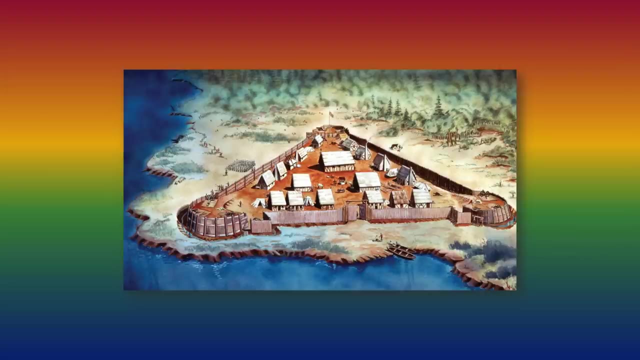 colony in the Americas, which is why Old Dominion is the state nickname today. After a rough start, the settlement of Jamestown, located on the north bank of the James River, eventually thrived as the first permanent English settlement in the Americas. They first 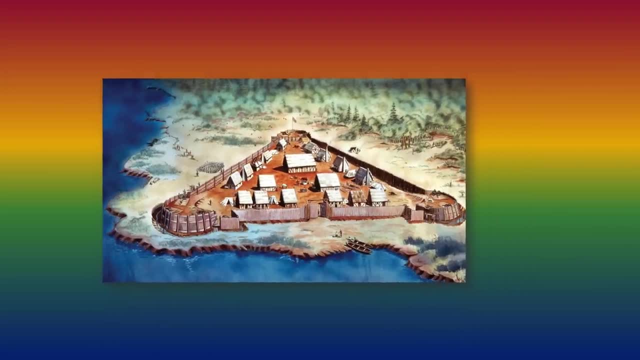 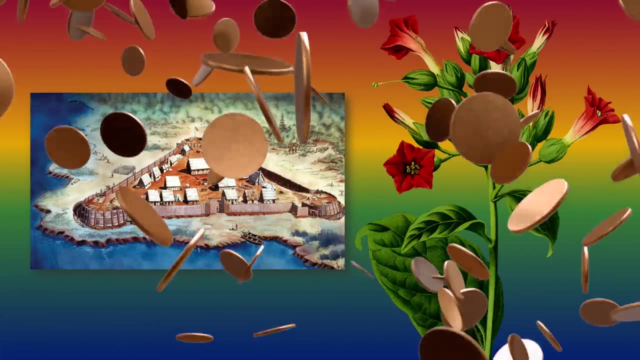 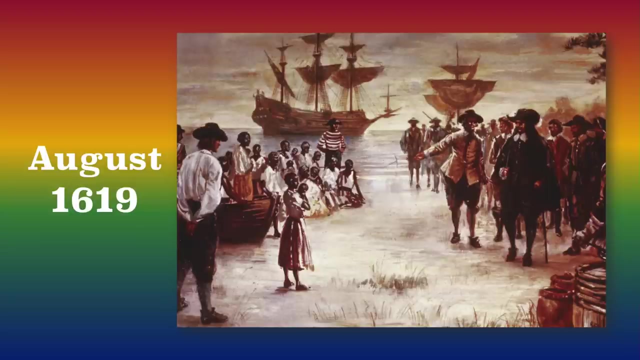 settled the area for gold, but ain't no gold around these parts? However, they soon figured out how to grow tobacco, which might as well have been gold, am I right, Since it became so valuable? European settlement steadily increased after tobacco became a cash crop In August 1619,. 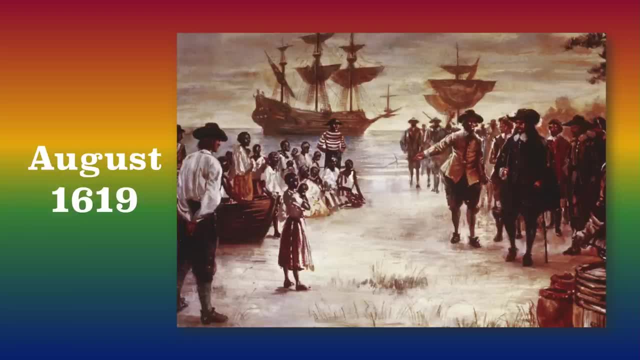 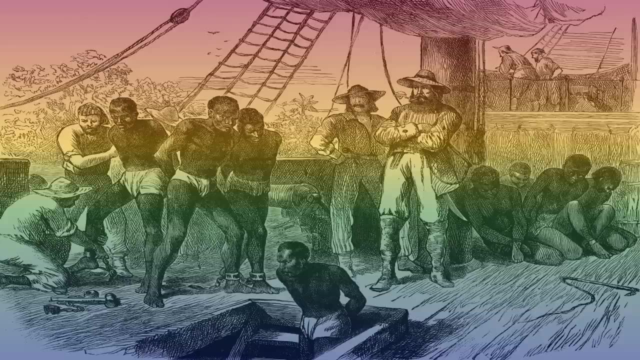 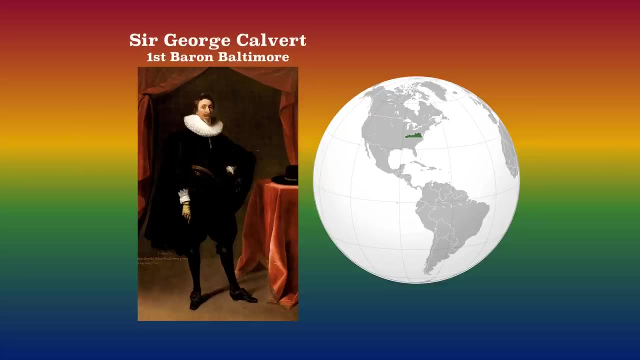 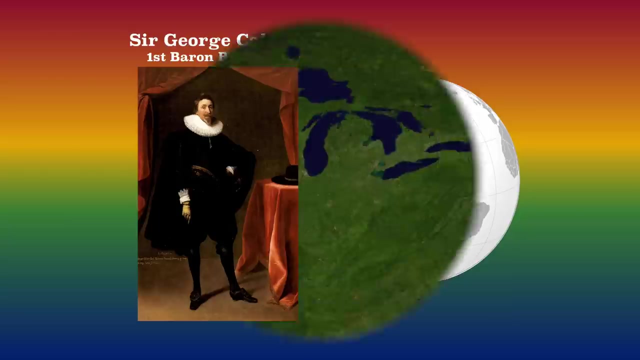 the first recorded slaves from Africa arrived near Jamestown and worked in tobacco fields. Over the following decades, more and more Africans would be forced to migrate to Virginia to become slaves. Meanwhile, a dude known as Sir George Calvert, 1st Baron Baltimore, took quite an interest in the English colonization of the Americas. 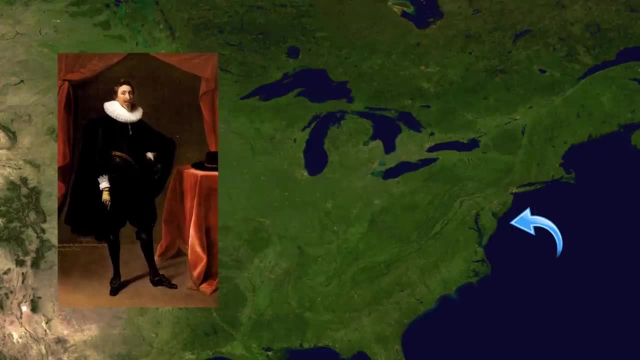 not only because he wanted to make money there, but also because he wanted to set up his own colony there as a place of refuge for persecuted Irish and Roman Catholics. See, I told you I would bring up Roman Catholics again. You didn't believe me, did you? 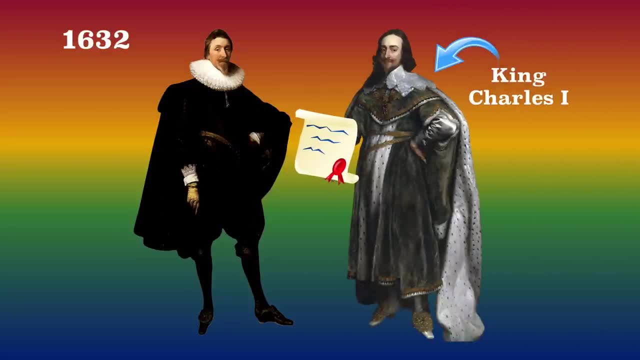 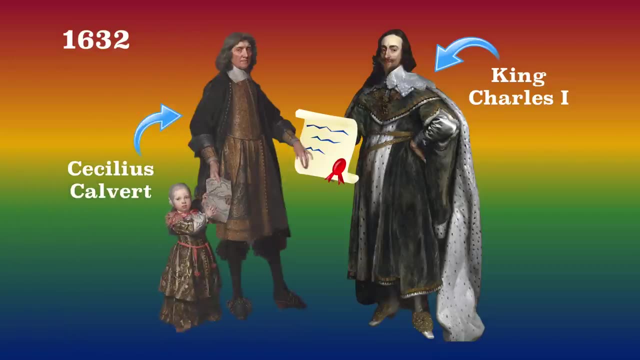 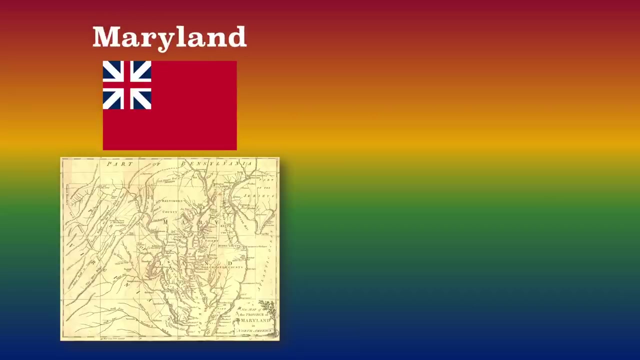 Anyway, in 1632, King Charles, I granted a charter to Calvert to form a colony, but then Calvert died, So his son Caecilius got it going with his other son, Leonard, becoming its first colonial governor. They named it Maryland and really pronounced. 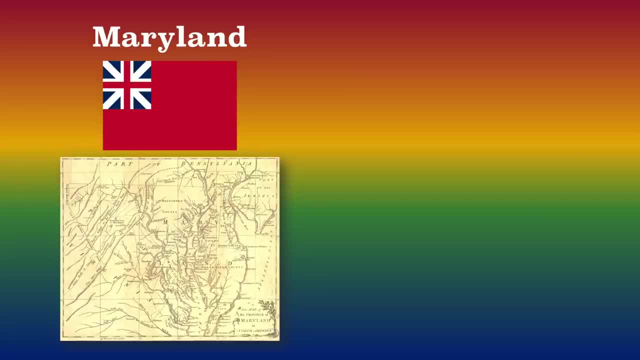 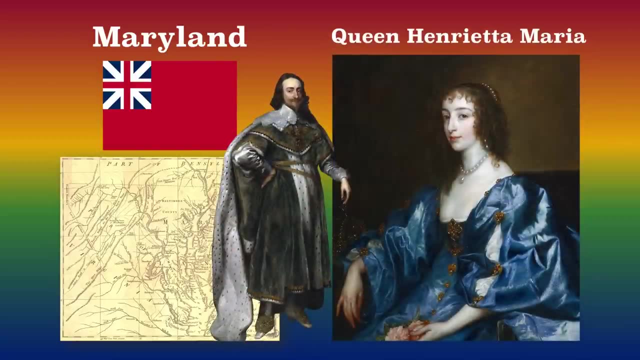 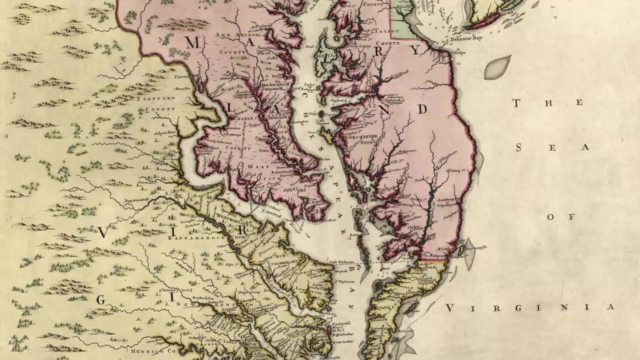 it that way, Not like us crazies today calling it Maryland. Besides, it was Mary's land. They named it in honor of Queen Henrietta Maria, the wife of King Charles. I Anyway, this began many, many years of border disputes between Virginia and Maryland. Many, 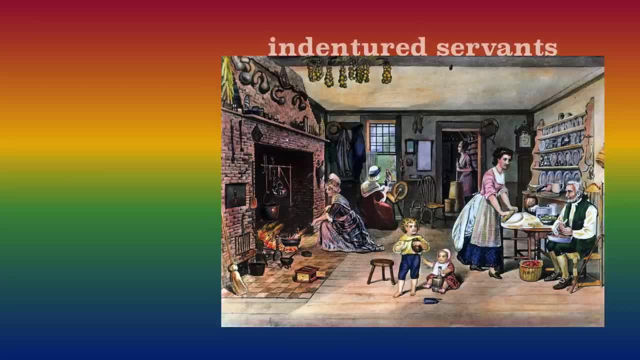 of the earliest settlers of the colonies of Maryland and Virginia were indentured servants or people who paid for their passage to the Americas by being forced to work for somebody for a certain number of years before getting their freedom. This really picked up after King Charles. I was- uh, you know- executed. 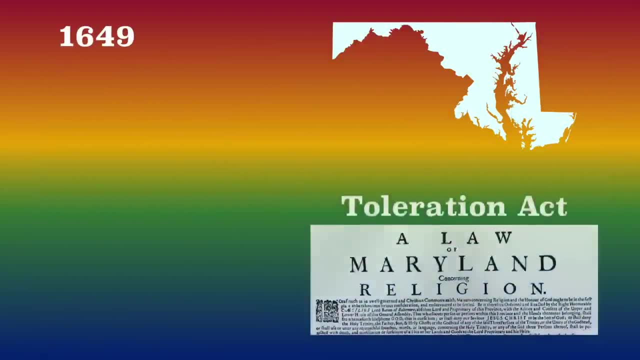 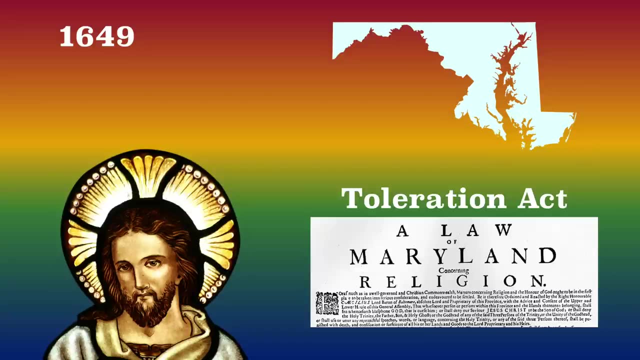 For treason in 1649, that same year, Maryland passed the Toleration Act, which kind of accidentally expanded religious liberty, even though it made it illegal to deny that Jesus was the Son of God, with the punishment of death. Holy crap. Still it was the first law on religious. 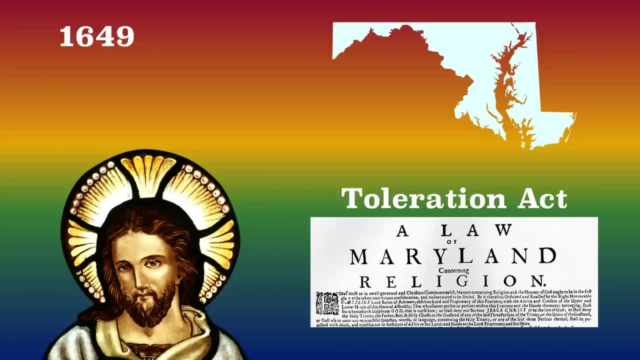 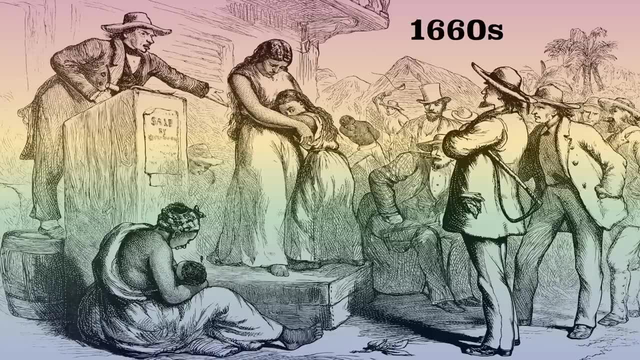 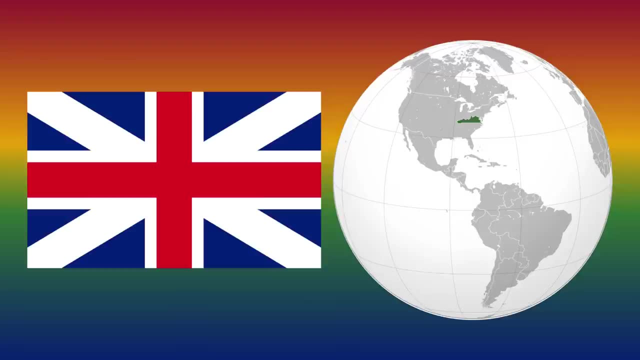 tolerance in British North America, so that's something Beginning. in the late 1660s, both Virginia and Maryland colonists would sadly pass new laws that further restricted the rights of all blacks, both free and slaves. Meanwhile the British Crown had taken over. 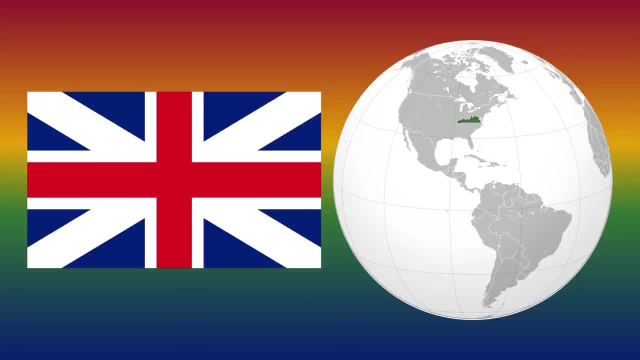 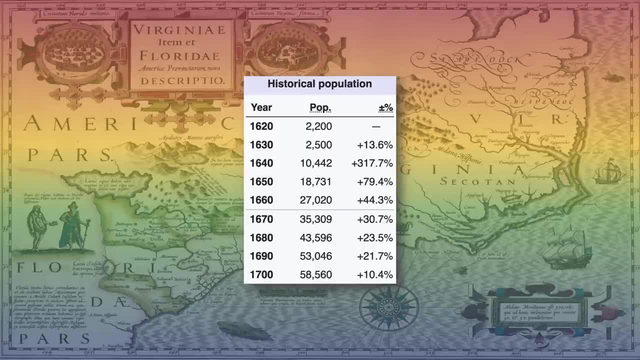 the colony of Virginia, since they didn't like how the London Company was running things. For the rest of the 1600s the colony grew quickly and brought a lot of wealth to England and certain plantation owners. In 1682, Maryland wanted to take over all the aforementioned 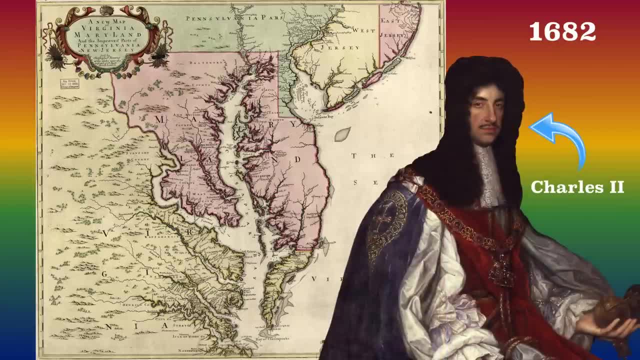 Delmarva Peninsula. but the new king, Charles II, didn't let them. instead giving what became the British Crown to the British. They were forced to leave the British colony and they were forced to leave the British colony. They were forced to leave the British. 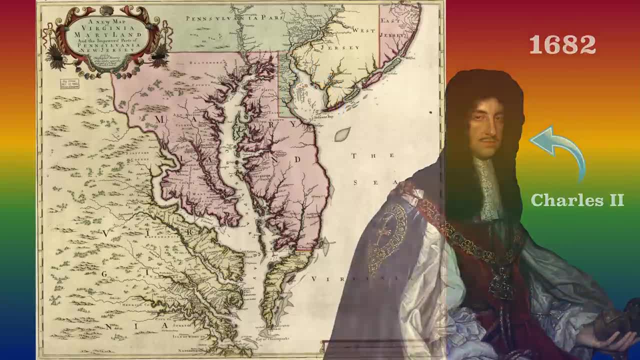 colony and they were forced to leave the British colony. They were forced to leave the British colony and they were forced to leave the British colony. They were forced to leave the British colony For the next 75 years or so. Maryland now had border disputes with Pennsylvania. 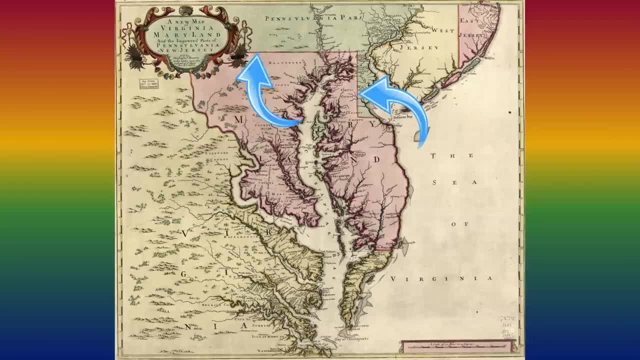 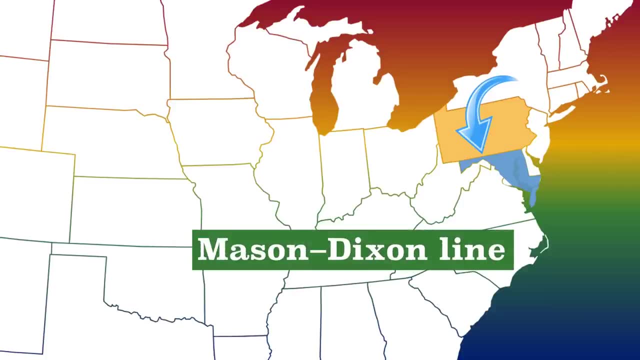 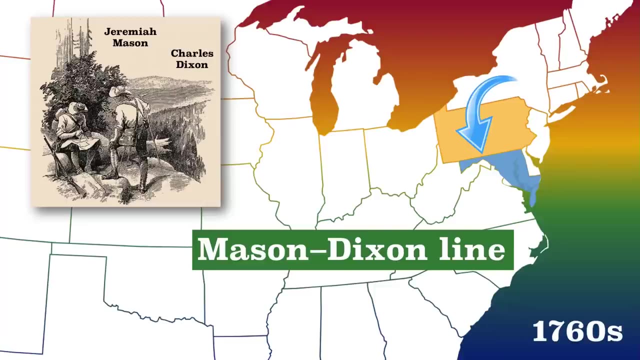 regarding both its eastern border and northern border. Wait, northern border, Yep, that's a pretty famous border. Today it's known as the Mason-Dixon Line, named after Jeremiah Mason and Charles Dixon, who drew it up. in the 1760s They settled the northern border between 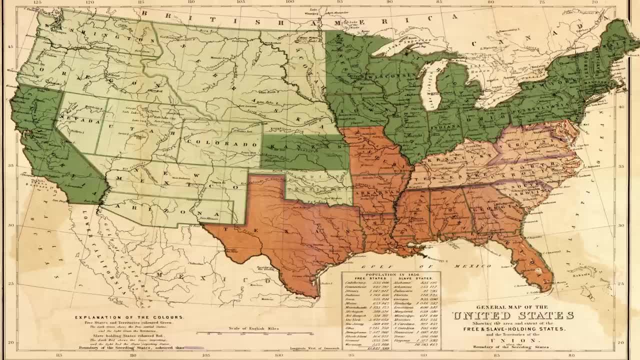 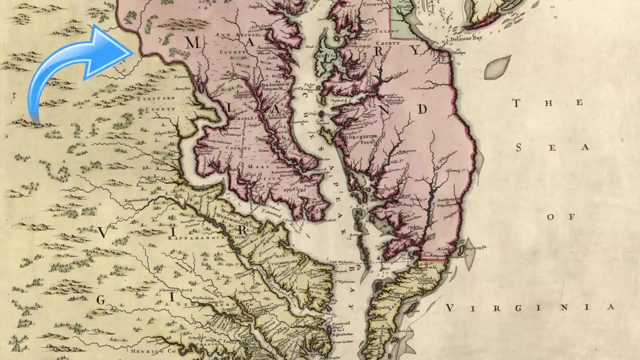 Maryland and Pennsylvania and they're now in the Northern Border. Maryland and Pennsylvania once and for all dadgummit, And that border eventually became an informal boundary between states in the north, where slavery was illegal, and states in the south where slavery was legal. Meanwhile, out west Virginia still had been disputing Maryland's. 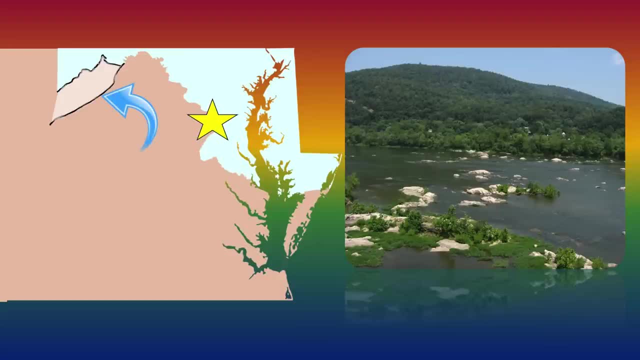 southern border. Maryland wanted it to be the southern branch of the Potomac River. Virginia wanted it to be the northern branch. Long story short. Virginia won the border battle since they were the bigger, more powerful colony. Virginia and Maryland did settle disagreements. 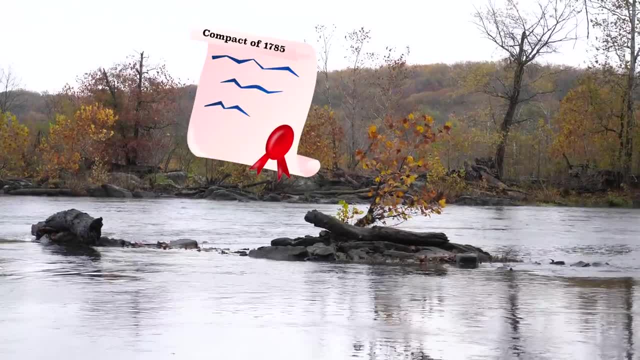 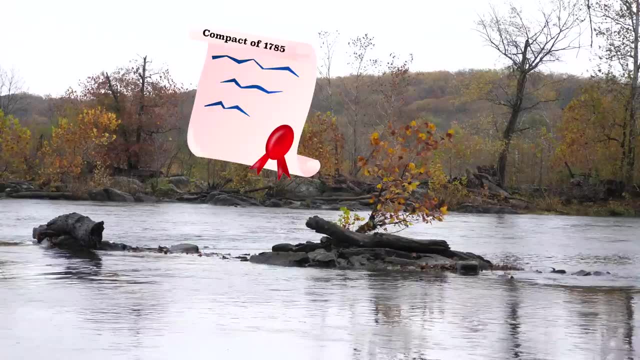 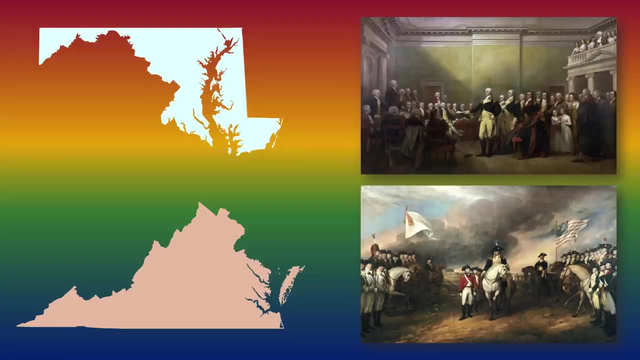 over how to share the Potomac River. However, with the Compact of 1785,, which served as a model for other states on how to settle disputes in the future, the citizens of both Maryland and Virginia played a big role, fighting for independence from Great Britain. Obviously, 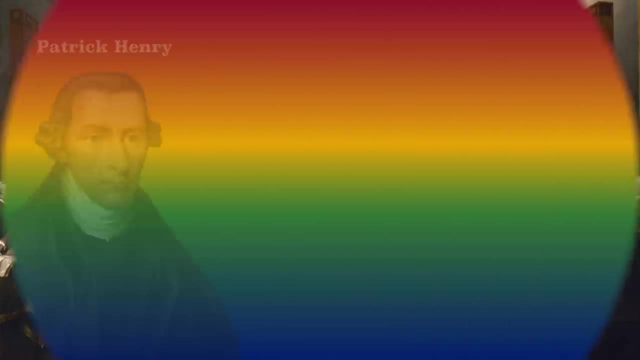 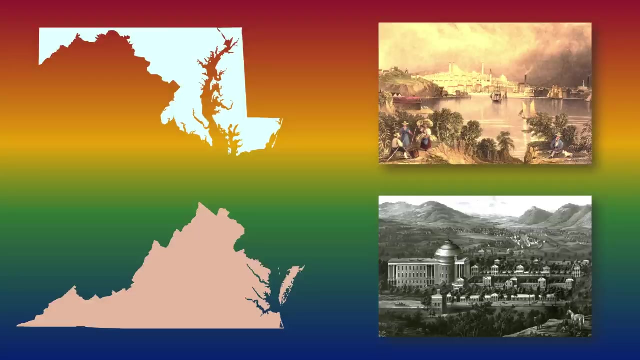 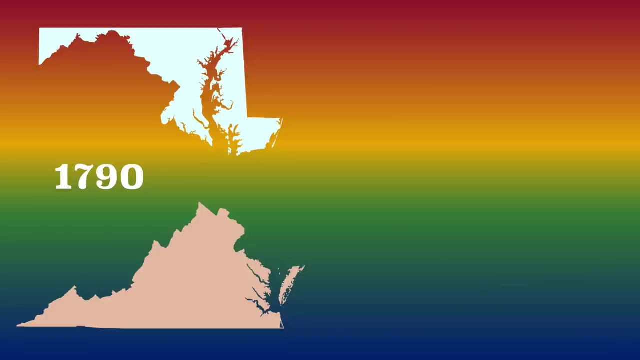 some of the most important figures from the Revolution, like Patrick Henry, Thomas Jefferson and George Washington, came from Virginia. After the United States became an independent country, both Maryland and Virginia thrived. In 1790, Virginia was the most populous state and Maryland was sixth most populous. 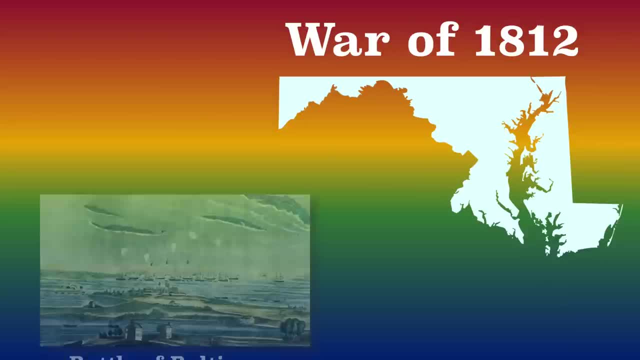 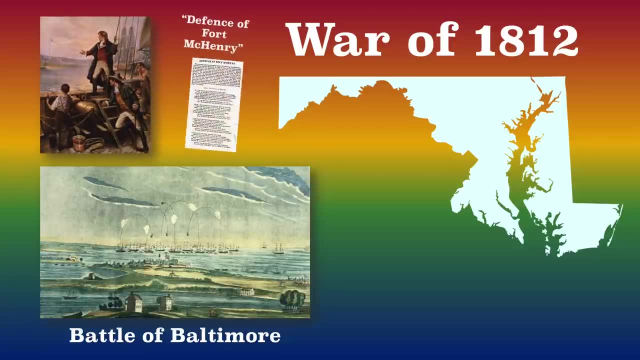 In the War of 1812, Maryland saw a lot of action, especially with the Battle of Baltimore at Fort McHenry. It was the battle which inspired Francis Scott, who was the key to write the poem Defense of Fort McHenry, which later became the lyrics: 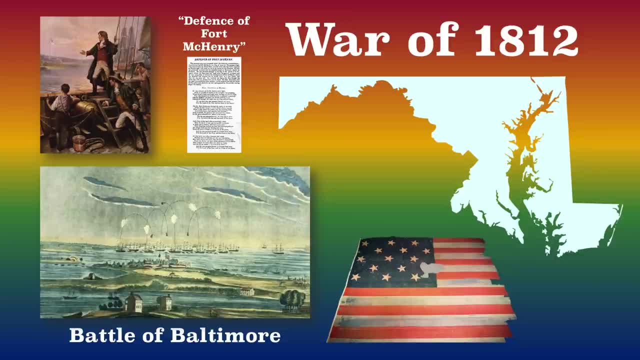 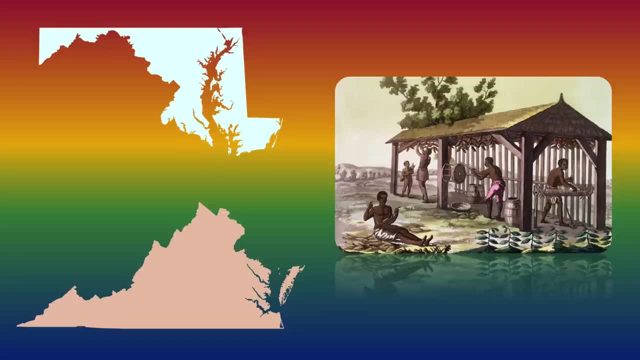 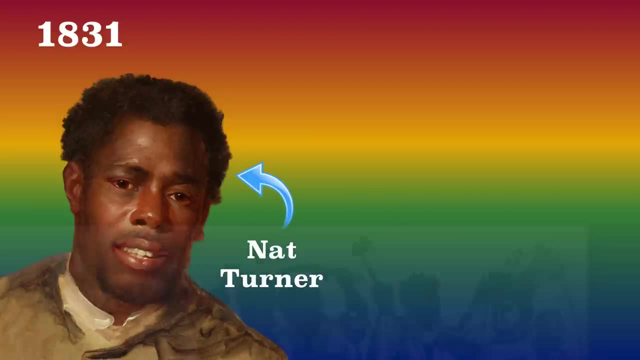 for the Star-Spangled Banner, which today is the national anthem of the United States. Sadly, a big reason why the two states thrived in the early 1800s was slave labor. In 1831, an enslaved preacher named Nat Turner led a slave rebellion in Virginia, killing as 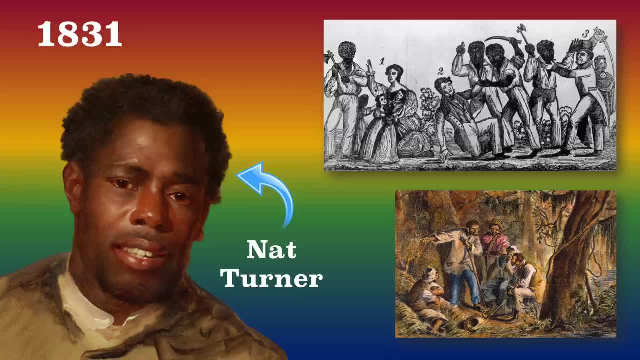 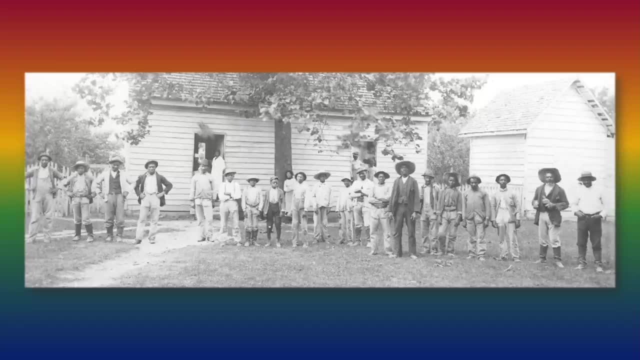 many as 60 people. In response, around 30 African Americans were hit by the ORFR. Americans were hanged or expelled from the state, and the General Assembly passed harsher slave laws, like laws making it illegal to teach slaves how to read or write. 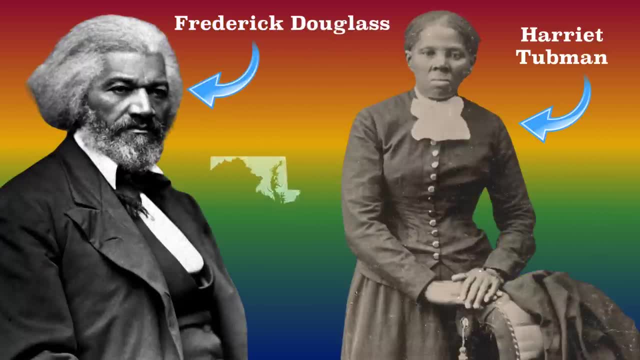 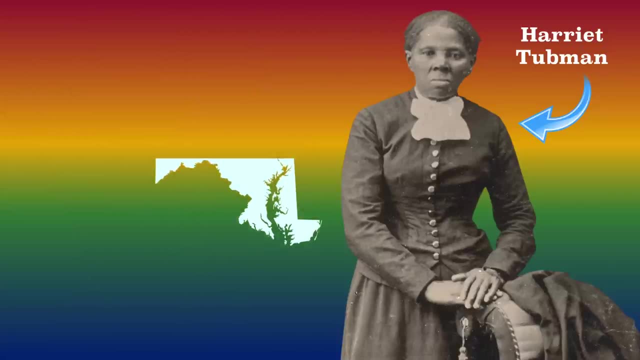 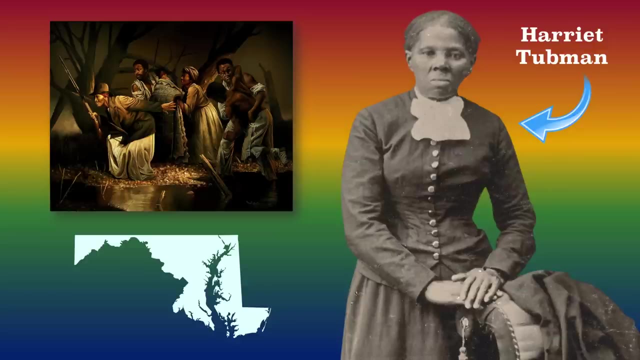 Both Frederick Douglass and Harriet Tubman escaped slavery in Maryland and both became heroes to the abolitionist movement. Tubman even went back to Maryland at least 13 times afterward to rescue at least 70 more people out of slavery. Dang, that's courageous. 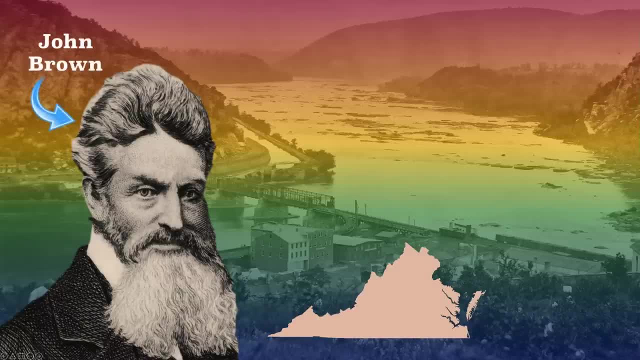 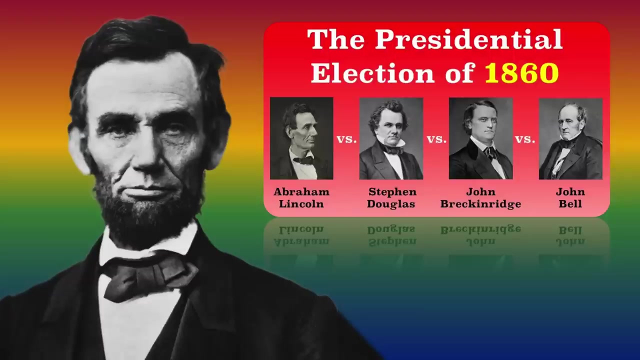 Virginia was also where the abolitionist John Brown tried and failed to incite another slave rebellion. in 1859. He attempted to take over a federal armory at Harpers Ferry, but ultimately Brown was captured and executed. After the election of Abraham Lincoln as President in 1860, Virginia's General Assembly voted: 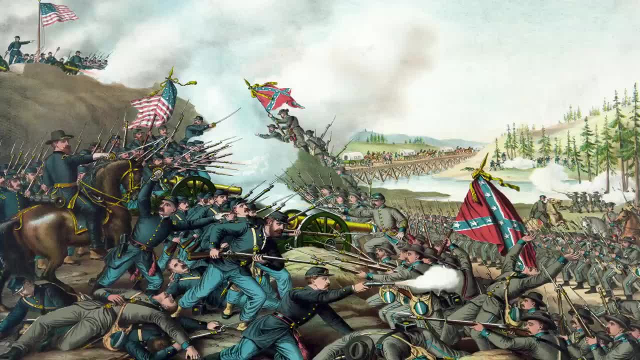 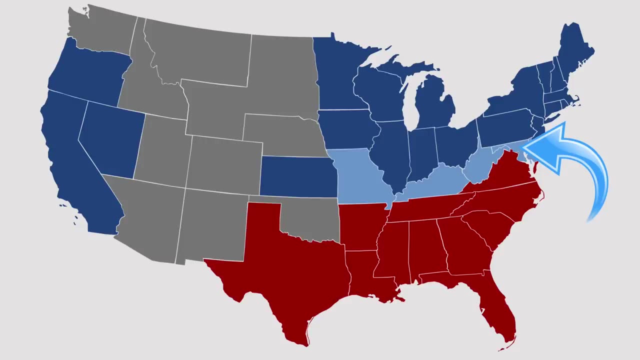 to secede from the Union over the slavery issue, And this soon. Virginia, along with other states seceding, led to the American Civil War, with Virginia leading the fight for the newly formed Confederate States of America. Maryland, even though it was still a slave state, decided to stay with the Union. 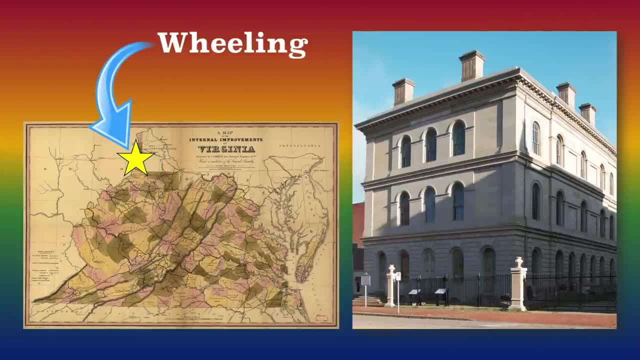 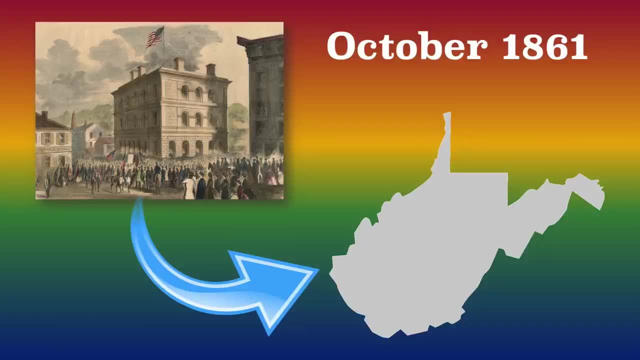 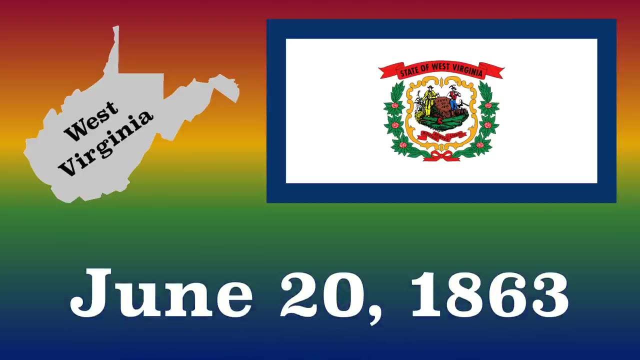 Meanwhile, several western Virginians in Wheeling also opposed secession and wanted to stay with the Union. In October 1861, they voted for a new state and the next April they had a new constitution. They were admitted to the Union as West Virginia on June 20, 1863. 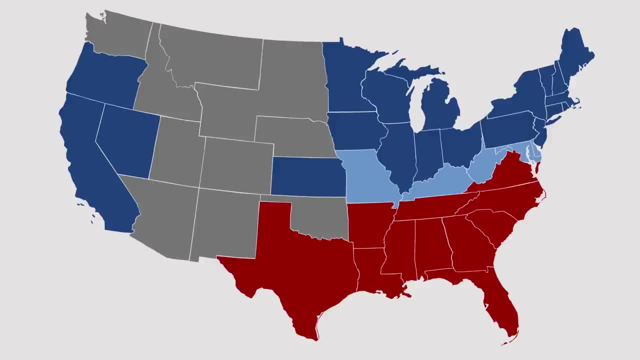 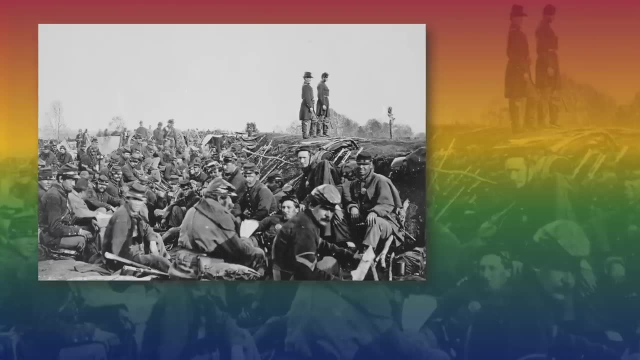 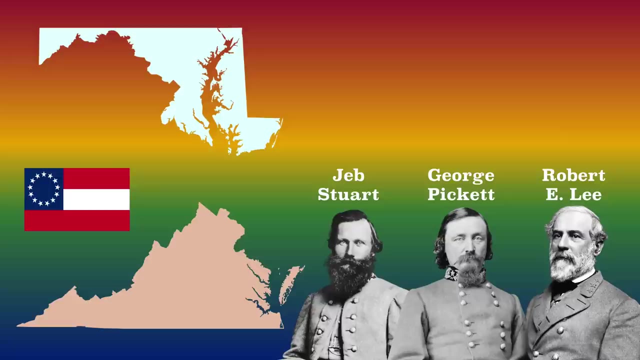 So this split Virginia into two states, with West Virginia fighting for the Union and Virginia fighting for the Confederates, And it was basically a smaller version of the entire war. Many big-name Confederate generals like Jeb Stuart, George Pickett and Robert E Lee, 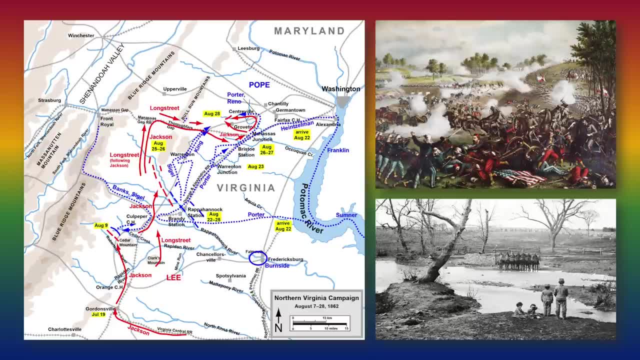 were from Virginia. Most of the battles in the Eastern Theater of the Civil War were fought in the West Virginia and most of the battles in the Eastern Theater of the Civil War were fought in the West Virginia. Most of the battles in the Eastern Theater of the Civil War were fought in the West Virginia. 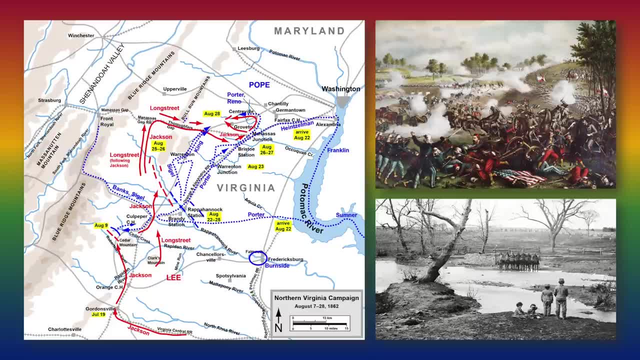 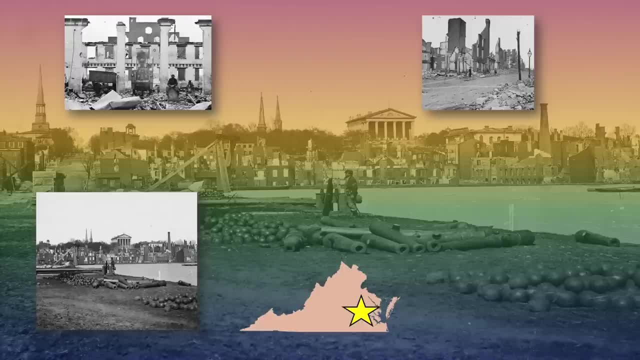 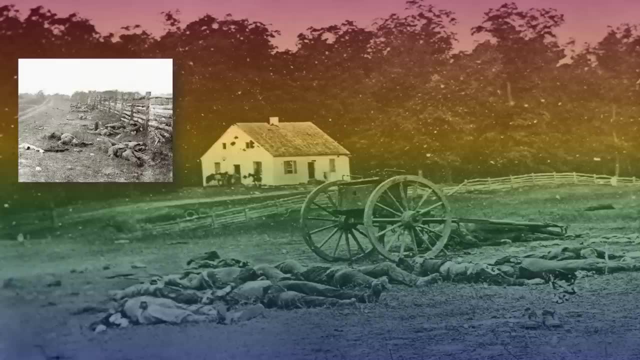 The Civil War took place in Virginia, mainly since the Confederates had to defend its national capital there, which was in Richmond. There is no doubt that the Civil War left Virginia devastated, although Maryland was where the horrific Battle of Antietam took place. 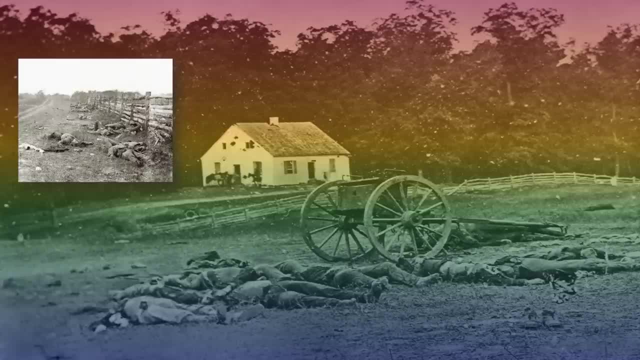 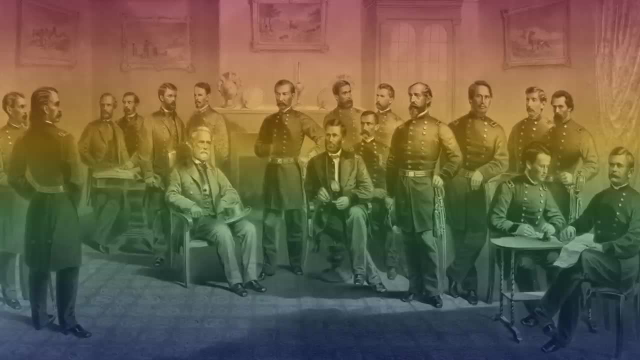 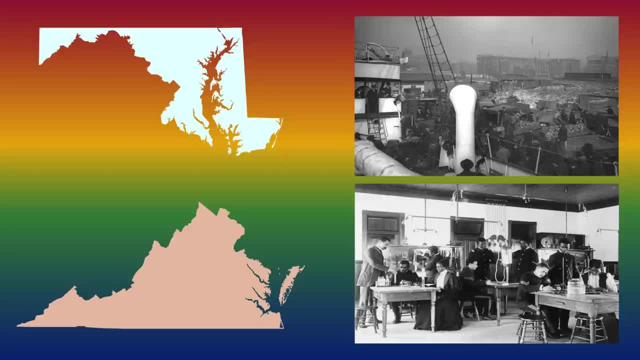 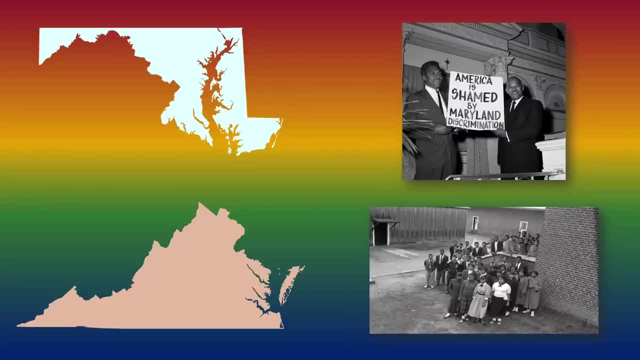 The Civil War was the day of the Civil War. The Civil War was the day of the Civil War. Virginia's economy struggled for the rest of the century. Maryland's economy did better. Racial segregation was also not nearly as pronounced in Maryland as it was in Virginia. 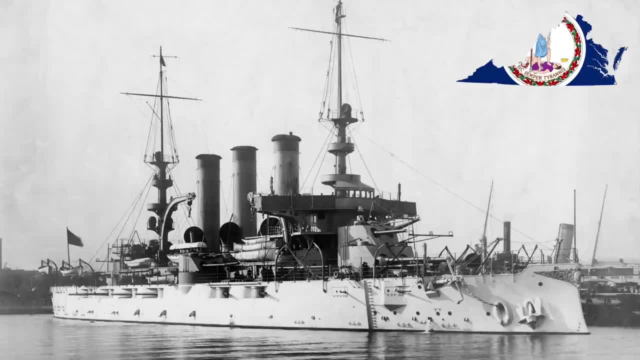 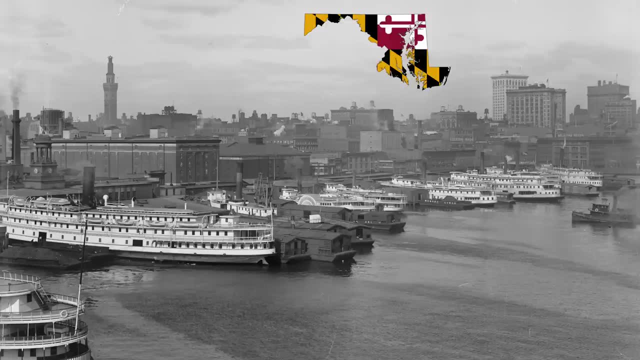 It wasn't until World War I when the economy really picked up again in Virginia. By that time, Maryland was booming, especially since it had attracted many more immigrants from around the world. For much of the 1900s, Maryland was growing at a faster rate than Virginia, but that trend 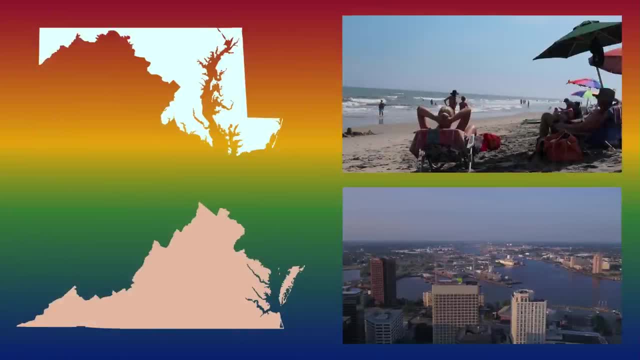 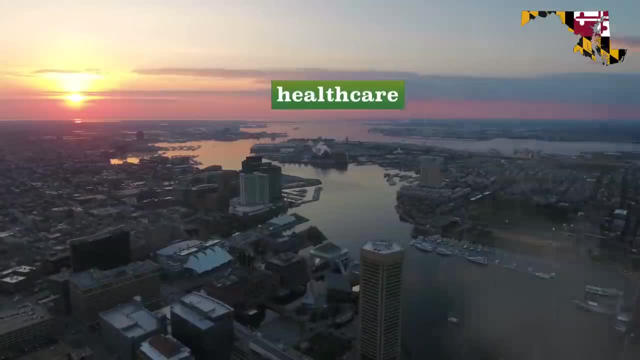 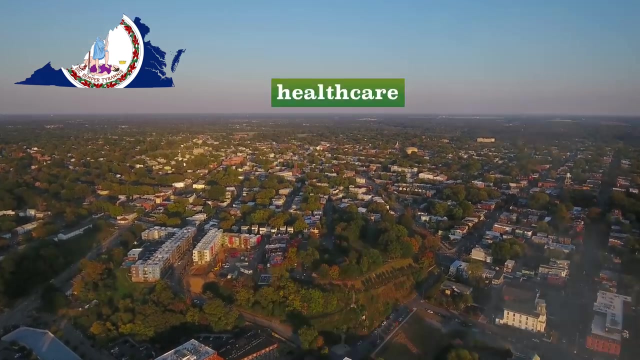 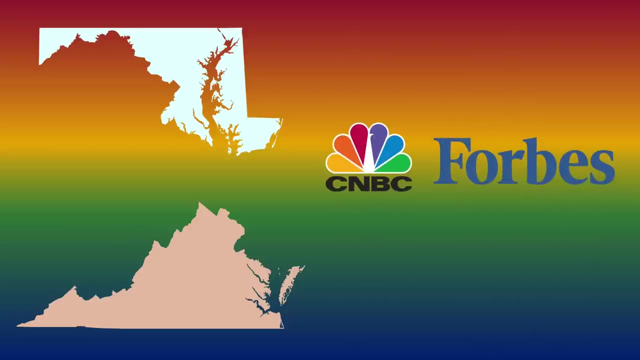 has reversed- reversed since the 1980s. Still today, the median household income remains higher in Maryland. Major industries today in Maryland include health care, government and public services and retail. Major industries in Virginia also include health care and government and public services, but additionally technology, According to both CNBC and Forbes Magazine. 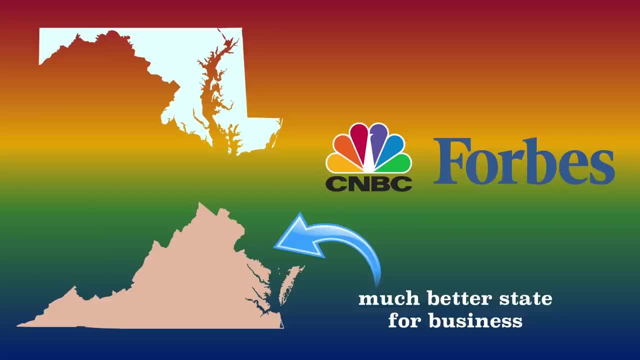 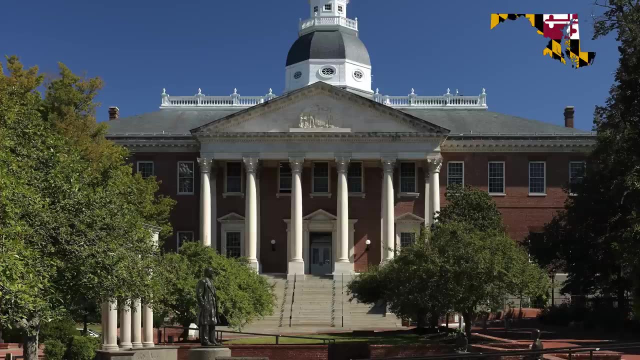 Virginia is a much better state for business. In fact, CNBC thinks Virginia is the best state for business right now in the entire country. And yes, you may not be surprised to hear that taxes are higher in Maryland. overall, More Maryland residents have college. 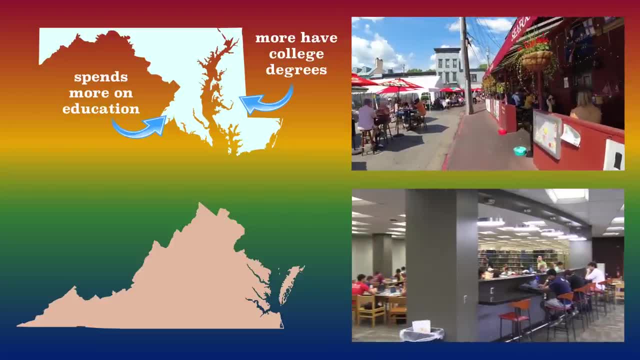 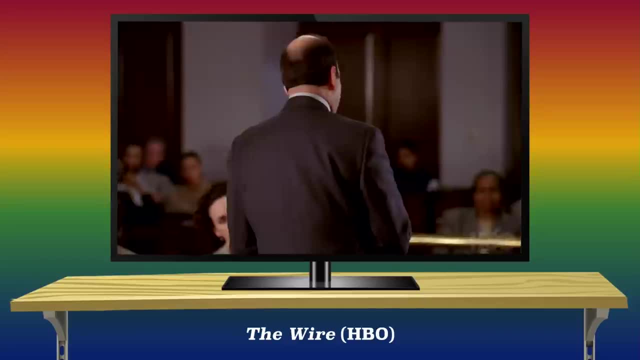 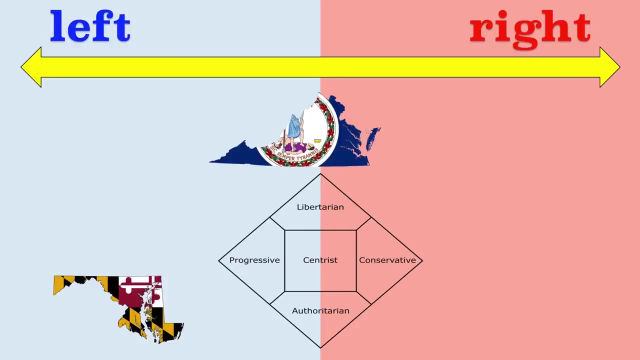 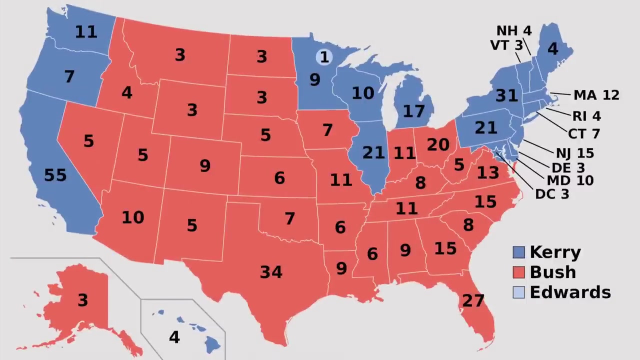 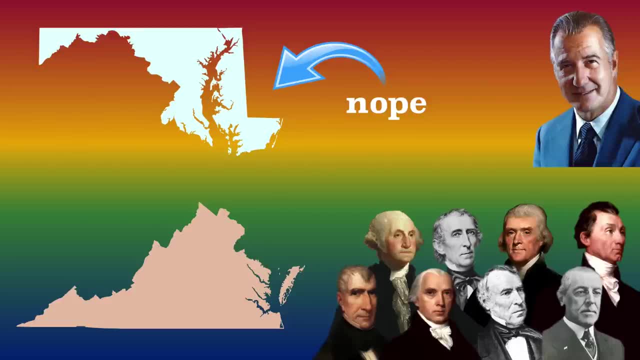 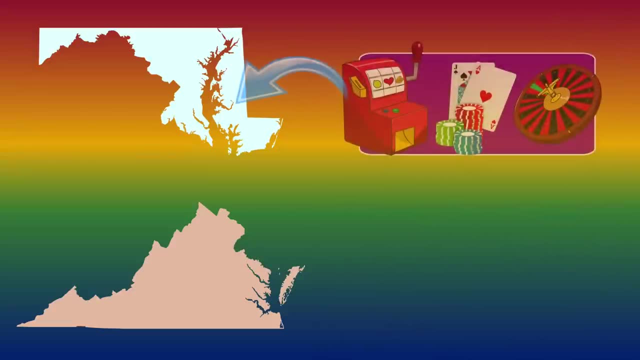 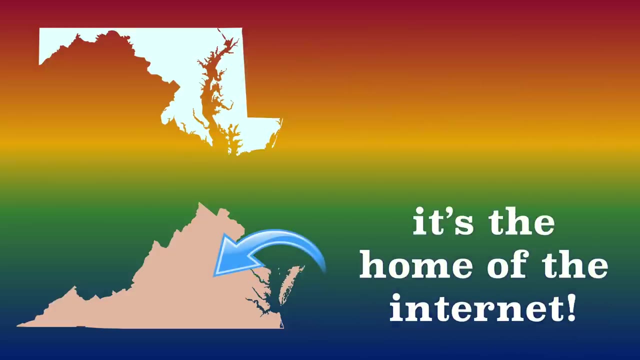 born in Maryland, surprisingly, although a vice president, Spiro Agnew, was from there, Not saying it's good to be proud of that. but you know it's much easier to gamble in Maryland. Here's something I learned only recently about Virginia: It's the home of the internet. 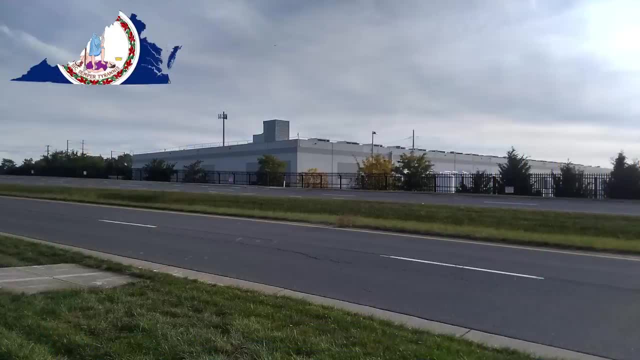 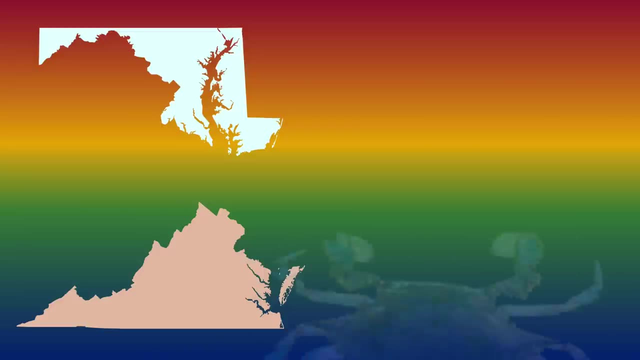 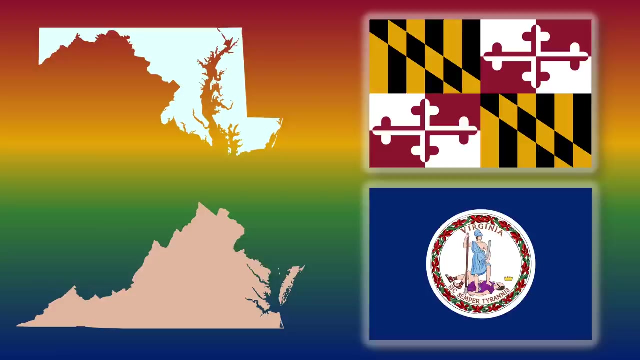 Well, it's the home of the majority of the world's internet traffic. Specifically, much of this traffic passes through the town of Ashburn, due to its many, many data centers. Maryland is known for its blue crabs and Virginia is known for its oysters. Maryland has a better flag, I don't care what. 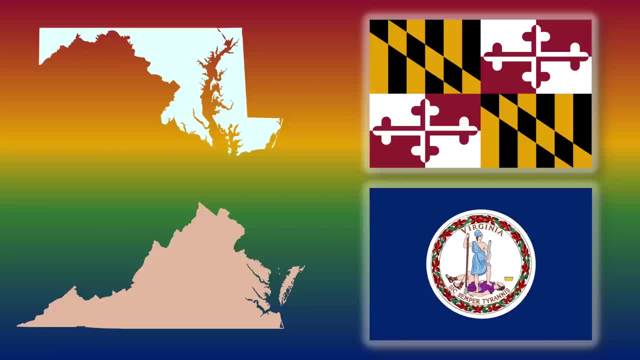 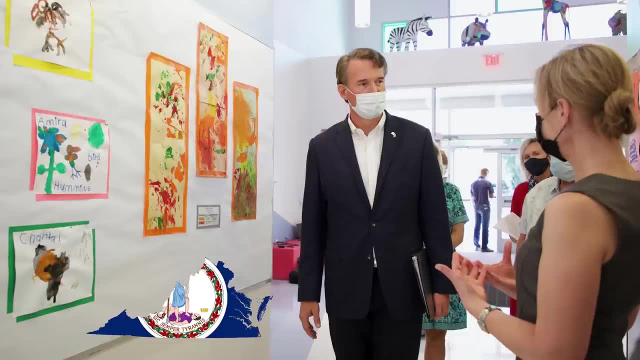 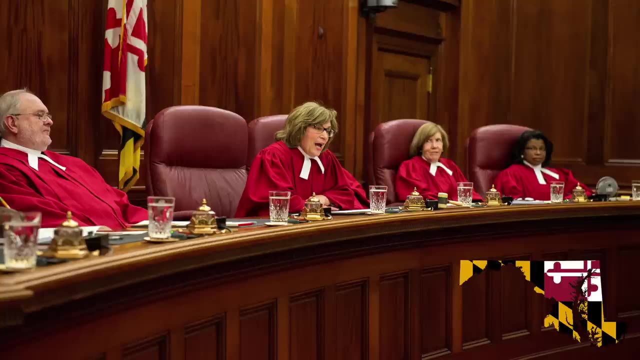 anybody says It's the coolest looking state flag in the country, Come at me. bruh Virginia is the only state in the country in which its governor can only serve one four-year term. I can dig that. Judges in the Maryland Court of Appeals randomly wear red robes. Okay. 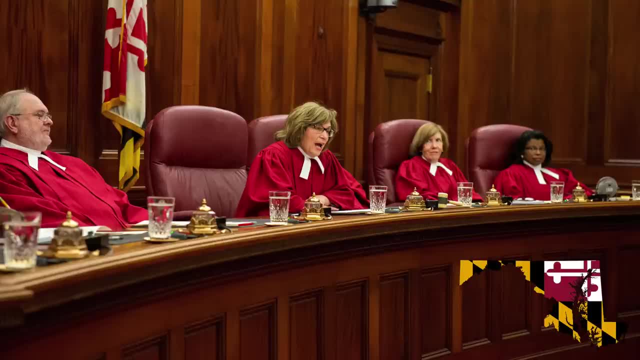 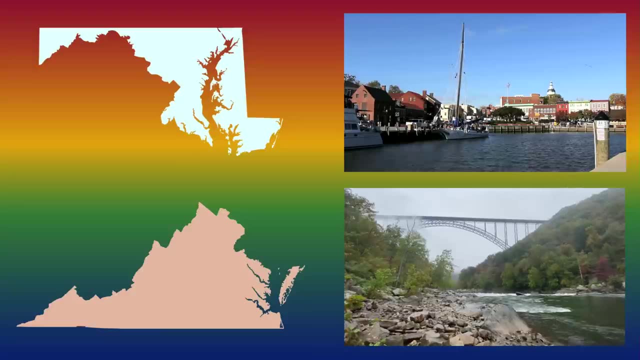 it's time to wrap this up, baby, because I'm talking about judge robes. In conclusion, Maryland and Virginia continue to be very desirable states to both live in and visit. They also remain two states where the North meets the South, and if you've never been, 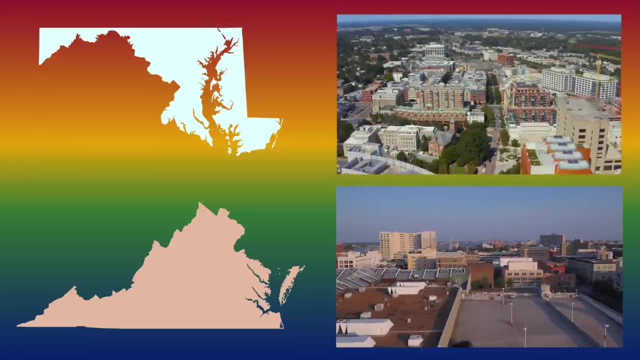 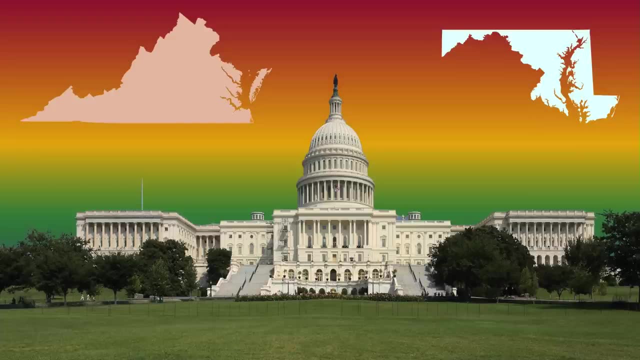 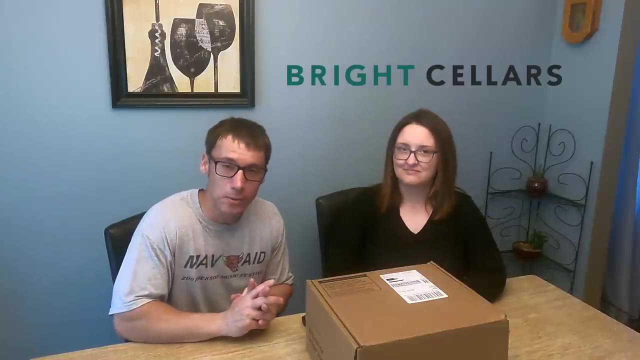 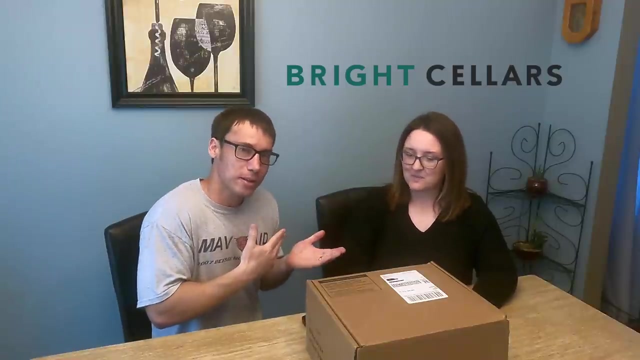 to the United States. it makes sense to visit these two states first to get a great sample of the country. Heck, you've even got the nation's capital between them. Thank you for watching. Have a great weekend and stay blessed. We'll see you next time. buh-bye. 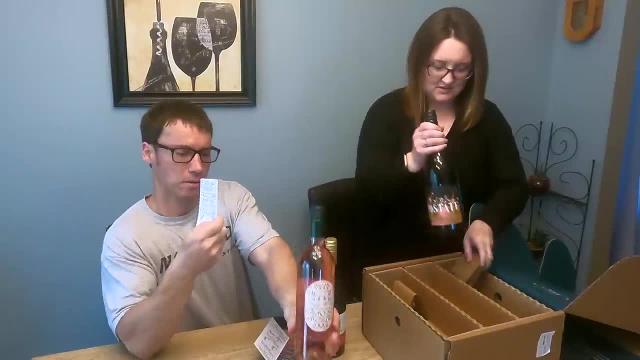 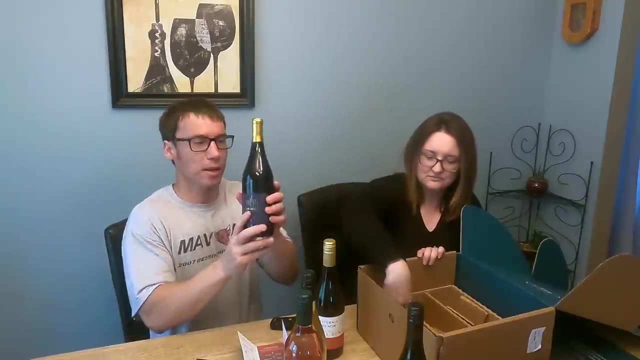 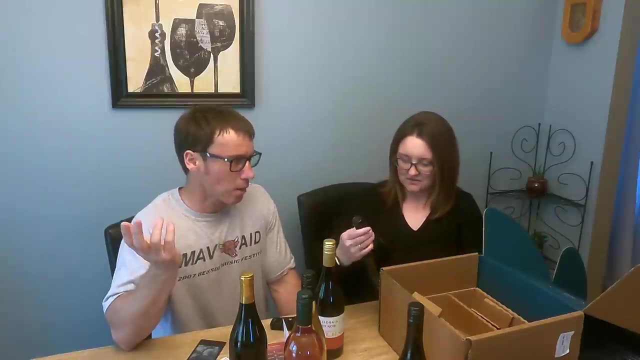 fettled press, apostate with a bunch of naked people on color, fast, it's a solemn rising tail, which is also a pinot noir. obscura, another zinfandel. which which of these wines are you most excited to try out? i want to try obscura. let's learn about obscura, so it says. 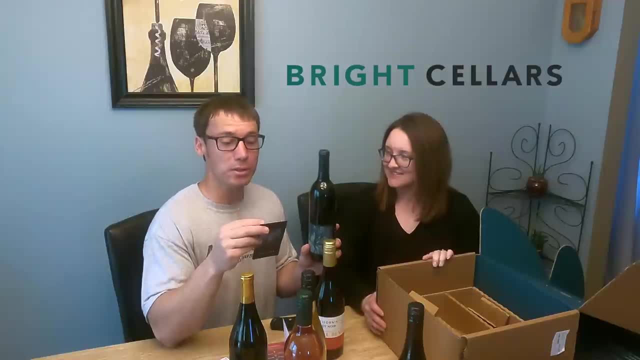 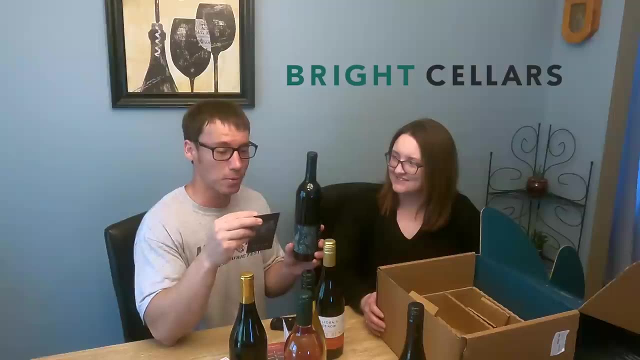 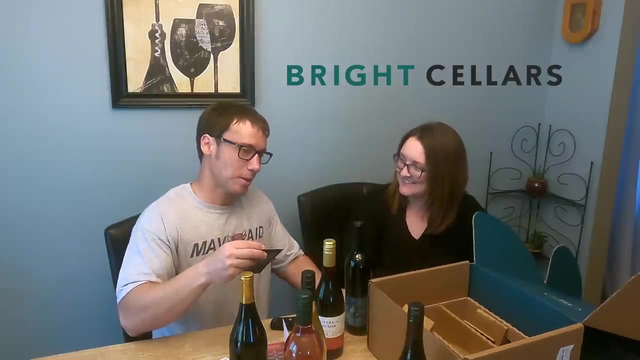 a classic california zinfandel. this wine is boosting with jammy strawberry and raspberry aromas, spicy black peppercorn and the palates is balanced by a ripe round mouthfeel. and you pair with watching the evening news. i don't think people watch the evening news anymore, but 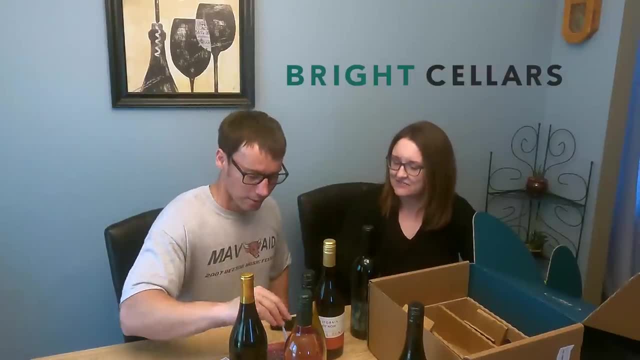 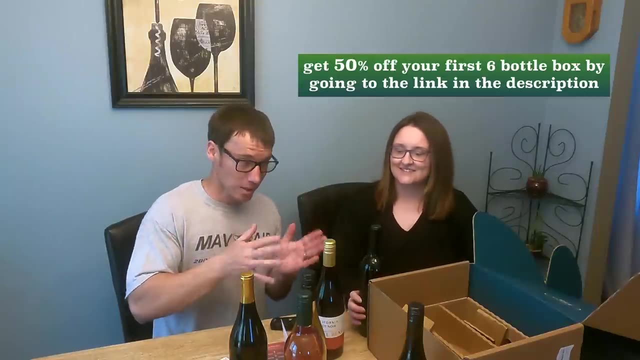 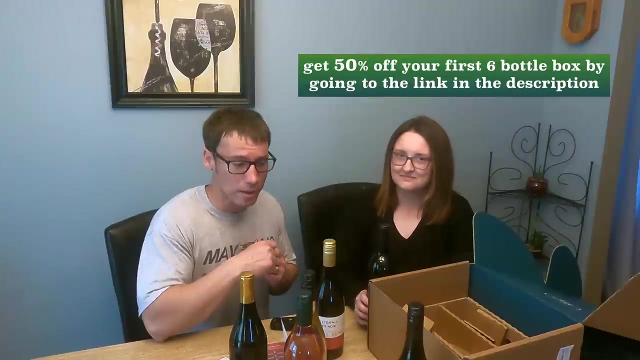 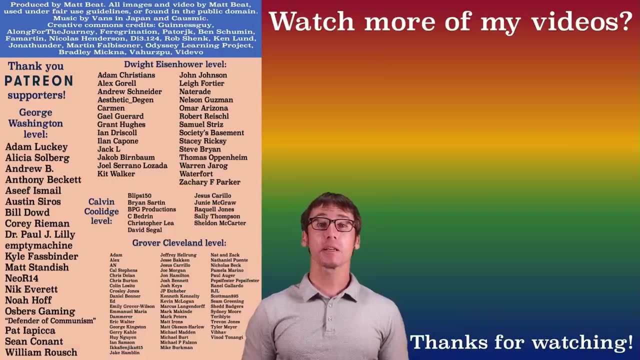 the evening youtube. how about that? the evening, mr beat? there you go, viewers of my channel will get 50 off. uh you. so which is better, maryland or virginia? a lot of you wanted me to compare those two states for this series, speaking of which i only have one state left, and that is michigan. what should i? 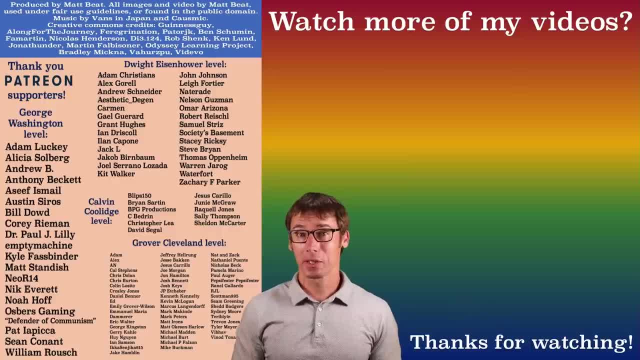 do with michigan. should i compare it to ohio, like many of my twitter followers suggested? or there's still the possibility of me comparing the upper peninsula and lower peninsula. let me know what i should do in those comments. i'm still torn between those two options. thanks for watching.